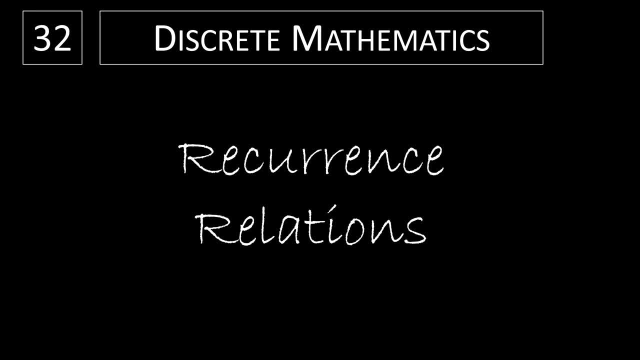 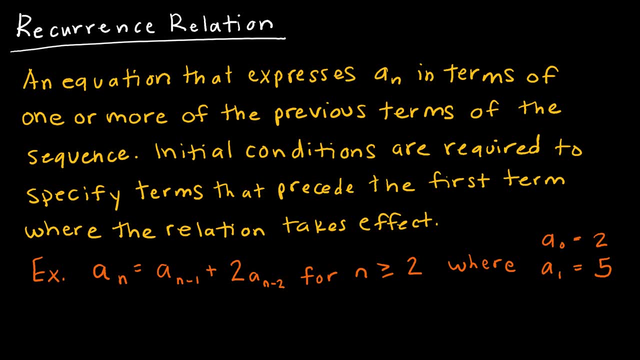 In this video, we're going to explore recurrence relations. A recurrence relation is just another way to express how to find the next values in a sequence, And a recurrence relation has two parts, and the first part is an equation, And so that equation is going to tell us how to get to the next term. 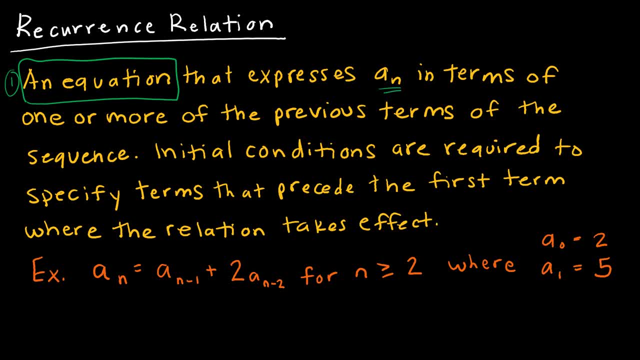 in the sequence And it expresses a of n in terms of one or more of the previous terms. So, like we said before, you need the term before it, or sometimes two terms before it, or three terms before it, in order to find the next term. So because 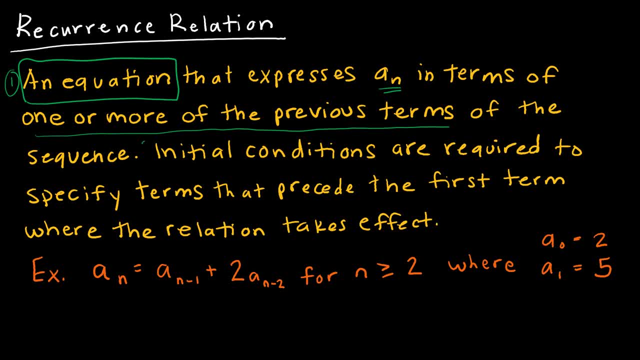 it's an equation that relies on previous terms. the second part of a recurrence relation is the initial conditions, And the initial conditions could be one previous value, some starting point, like a like we had for our arithmetic or geometric sequences, or it could be that they've also given us a sub 1, which 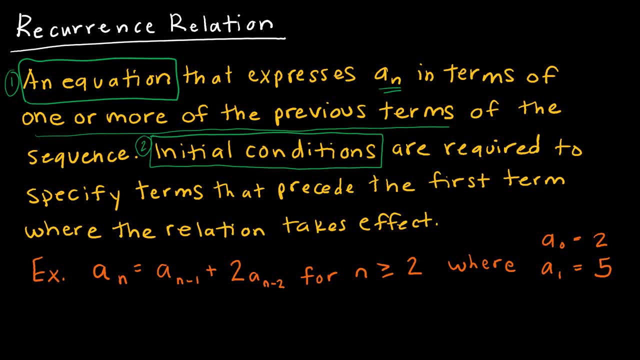 would be the next term in the sequence, And however many initial conditions you have will be based on your equation. So let's take a look at this example so you can see what I'm talking about. So, for my example, I have an equation and I 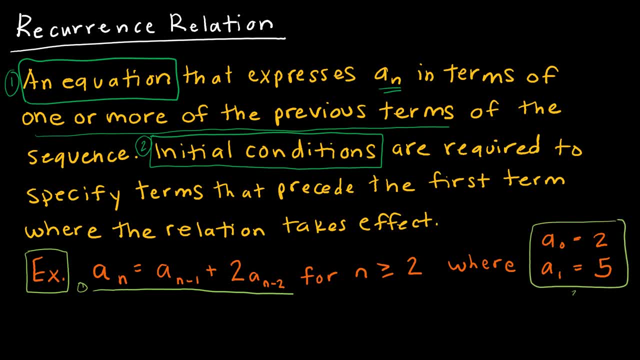 have initial conditions. And it also tells me the equation only works for n is greater than or equal to 2, and that's because over here I've given you a sub 0 and a sub 1.. So they're saying this function starts at a sub 2.. So that's. 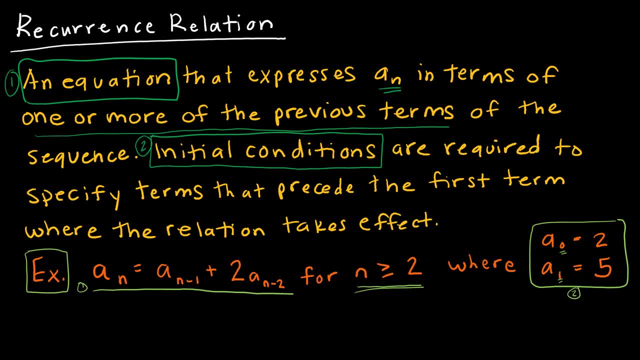 what my recurrence relation is. So that's all of the parts of my recurrence relation. Here's how it works In this case. we're looking at a recurrence relation to find the next term in the sequence. So let's take a look at this. 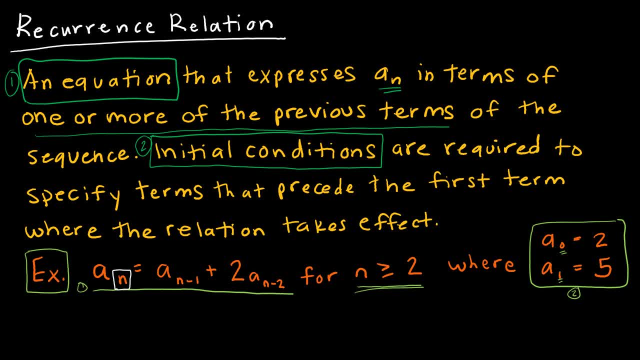 example. So here's how it works. So let's take a look at this example. So let's find whichever term I want. I have to take the term before it: n minus 1,, a sub n minus 1, and two times the term before that. So that's why I have two initial 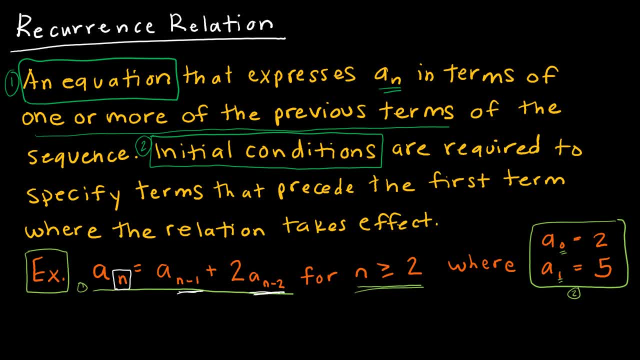 conditions, because my next term is based on the values of the two terms before it. So we already know a sub 0 is 2.. So again, if I wanted to write this in a sequence, the first term is 2,, the next term is 5.. So I'm going to take a sub 0,. 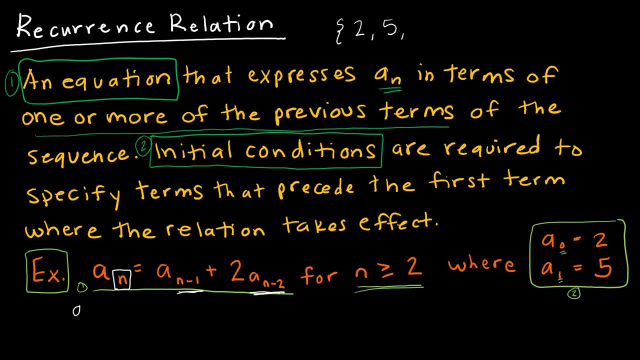 and if they said, hey, find some more, well then I have to do some math. So to find a sub 2, then I would take a sub 1 plus 2 times a sub 0, according to this equation, So a sub 2 is a sub 1, or 5, plus 2 times a sub 0,, which is 2.. So 5. 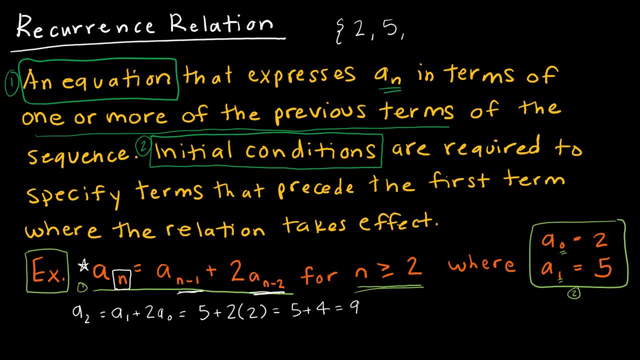 plus 2 times 2 is 4, gives me 9.. So that's why I have two initial conditions. that means my next term would be 9.. A sub 3.. A sub 3, again according to this equation says: take a sub 2 plus 2 times a sub 1.. So a sub 2, I just found that. 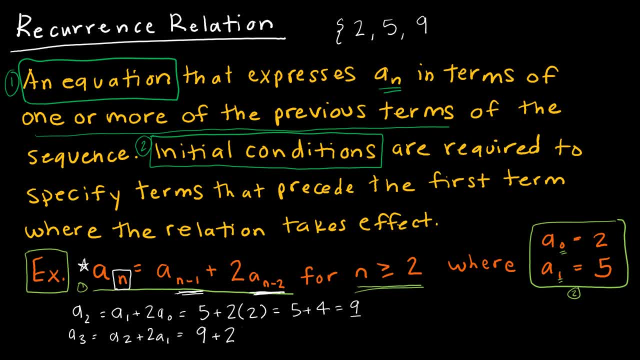 was 9.. 2 times a sub 1 would be 2 times 5.. So 9 plus 10,, which is 19.. We can see that we could keep continuing this. So a sub 4 would be a sub 3 plus 2 times. 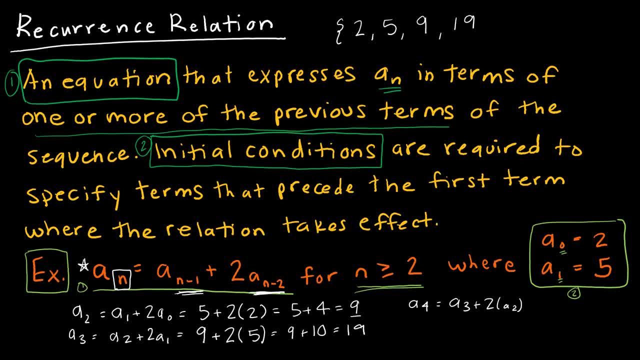 a sub 2.. And that would be a sub 3 is 19.. 2 times a sub 2,, which was 9,, which gives me 19 plus 18,, which gives me 37. And I'm not going to keep going because 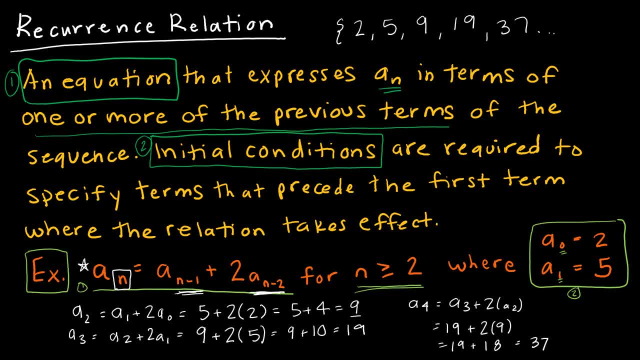 obviously, oops, we can see that we have a sub 3 plus 2 times a sub 2, which is 20 times a sub 2 plus 2 times 5.. So a sub 3 plus 2 is about 10.. And the thing? 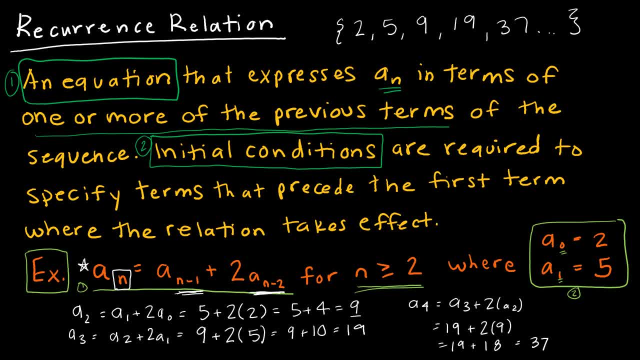 that keeps going is a sub 3 plus 2 plus 2 times a sub 2 minus 4 times a sub 2 plus 4.. So a sub 3 plus 2 plus 2 times a sub 2 plus 2 is less than or equal to 2 times. 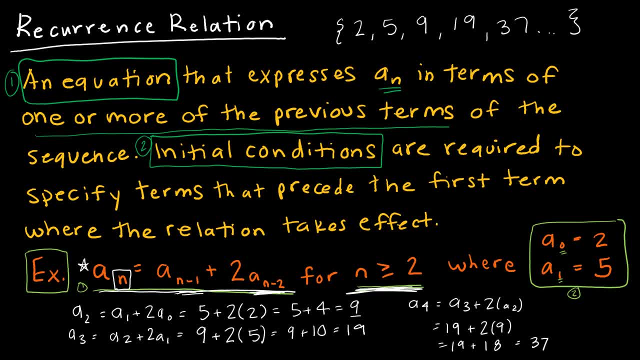 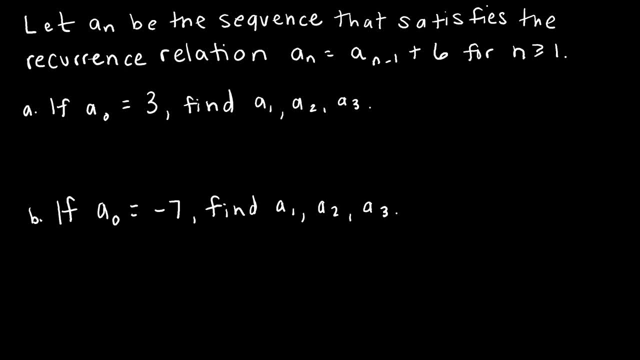 a sub 2 plus 2 times a sub 2 plus two. So that's the first one. Now for a second question. So you're wondering: if you had a dipole, what would it be? So the answer is, again, that's a real question. So if I were to give a 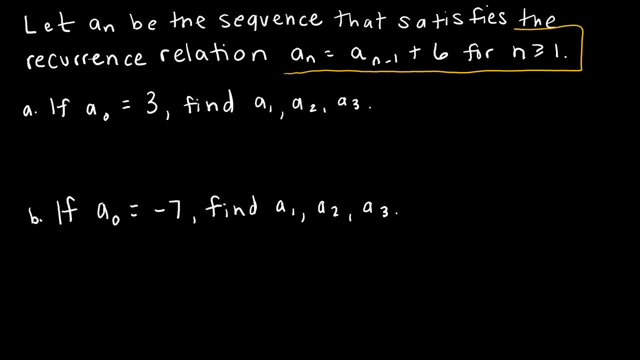 step of two seems to give you more or less meaning. So you have a drop and a drop, And what I'm going to do is I'm going to do a little bit of an sequence. I just take the previous term and I add six, and that is for n. greater than or equal to. 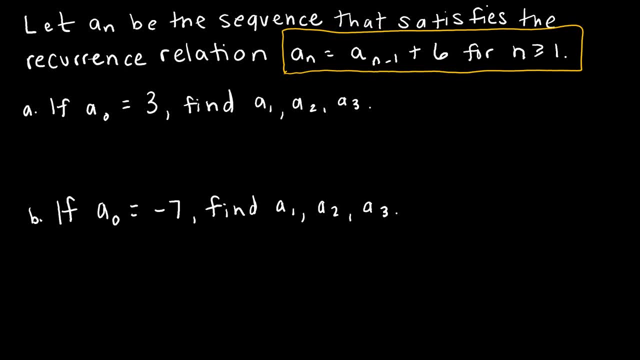 one, which means, of course, that they're going to give me a sub zero and then I'm going to need to find the rest of them. So, looking at this, we're saying to find, we have a sub zero To find. 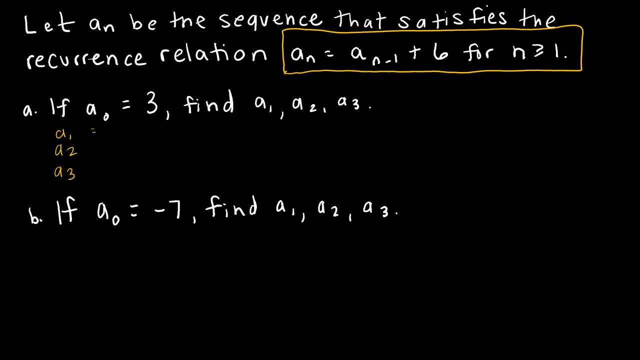 a sub one, a sub two, a sub three. that's what we're asked to find. To find a sub one, I'm going to take a sub zero plus six. To find a sub two, I take a sub one plus six To find a sub three. 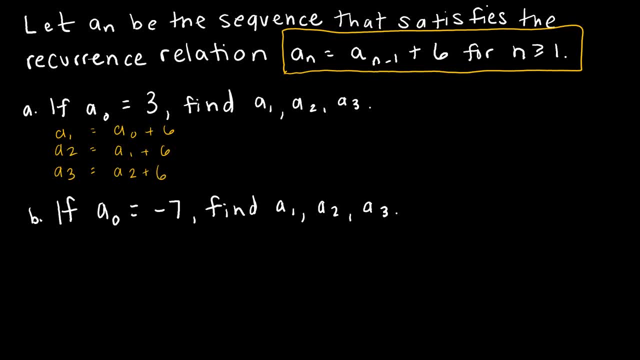 I take a sub two plus six. So a one is a zero, which is three plus six, which is nine. A two is a one, which is nine plus six, which is 15.. And a three is a two, which is 15,. 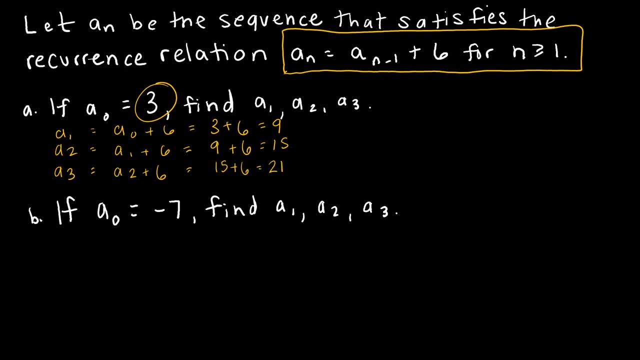 plus six, which is 15.. Now this is, as you probably recognize, because we talked about arithmetic and geometric sequences. this is just an arithmetic sequence. All I'm doing is just adding six to get from one term to the next, So I'm getting ahead of myself. but this, if you'll recall, could be written: 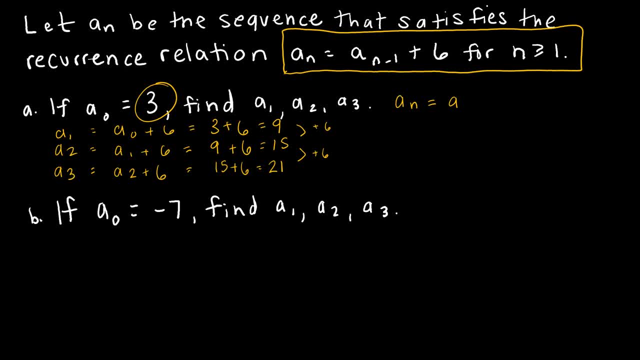 as an arithmetic sequence, where arithmetic sequence was a plus d n. So in this case I could write a sub n as a, which is three plus my common difference of six n. Now again, this is not necessary for this question. The reason that I bring it up is: 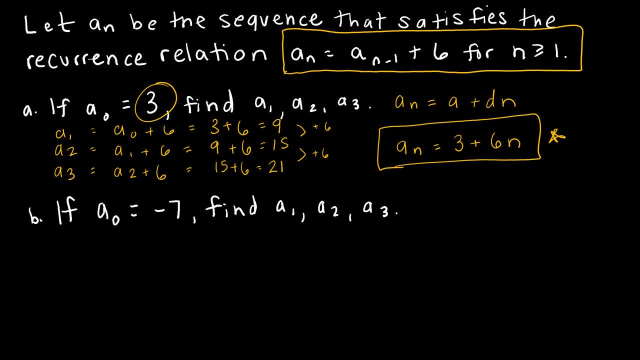 because recurrence relations are fine. but what if I said, find a 100?? Well then, to find a 100, I would need all of the values before a 100. So I would need all of the values before a 100.. 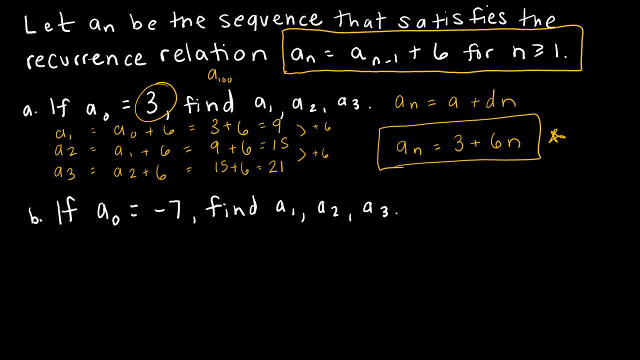 So I would need all of the values before a 100.. So I would need all of the values before it, because it's always based on the value before it. So if I don't want to find a four through a 99, in order to find a 100,, if I can write it in a closed equation like this explicit form: 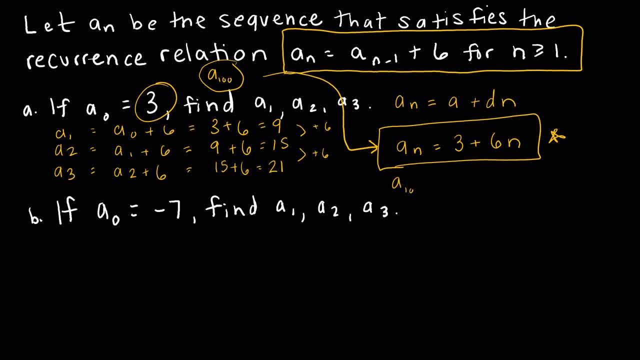 as we talked about before. then it's pretty easy for me to say: well, a 100 is three plus six times 100, which would be three plus 600, or 603.. So again, I'm kind of getting ahead of myself, but I just want you to see the relationship between 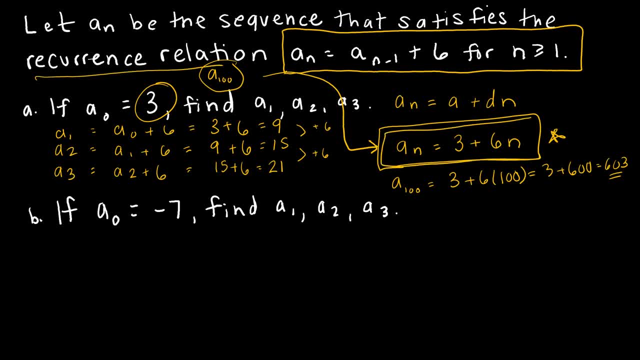 a recurrence relation and some closed form equation like this. So let's look at the second part of this. This is saying: hey, use that same recurrence relation that I gave you with the different initial condition, this time of negative seven. So again, I'm still saying a one, a two. 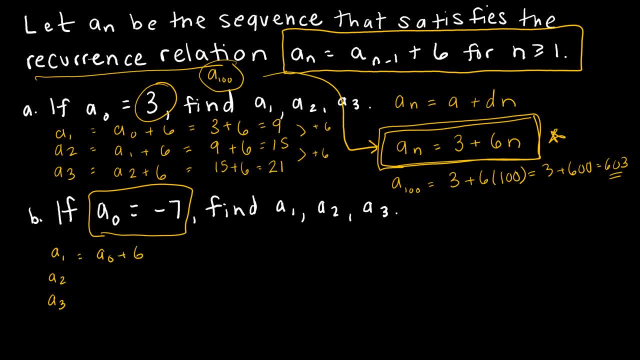 a three would be a zero plus six, a one plus six, a two plus six. I'm sorry, Yeah, that's right. I think I was confusing myself for a minute, But in this case a zero is negative seven, So negative seven plus six is negative one. 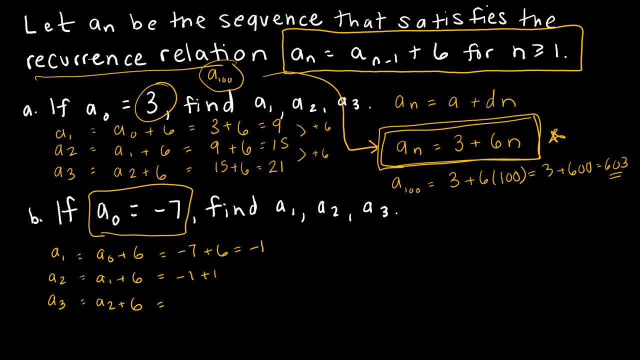 So a one is negative, one plus six is five, And then a one is five plus six is 11.. So I still have this common difference of six. So I still have this common difference of six. So if I wanted to, I could write this in the same format, but instead of three, three is replaced by negative seven, But it still has the six n. 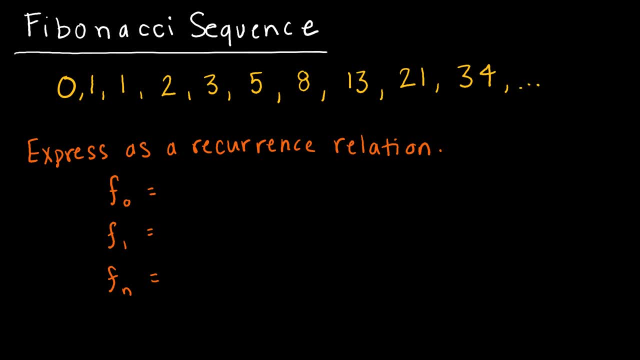 Let's take a look now at a very famous sequence that I'm sure that you've heard of, which is the Fibonacci sequence, And you probably know that a Fibonacci sequence, the next number is found by adding the two numbers before. So 01 added together gives me zero plus one, which is one. 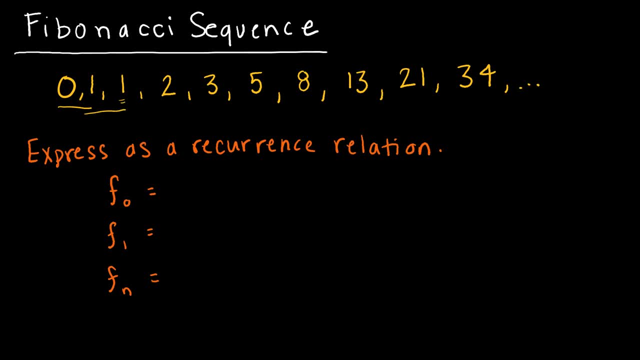 That's where this number came from. And then one plus one added together gives me two. And then one plus two added together gives me three. And then two plus three added together gives me five. So you knew all about recurrence relations even before you knew what you knew. But that's what a Fibonacci sequence is all about. So if we want to express this as a recurrence relation, all we would have to do is again include the two parts, which is the equation. 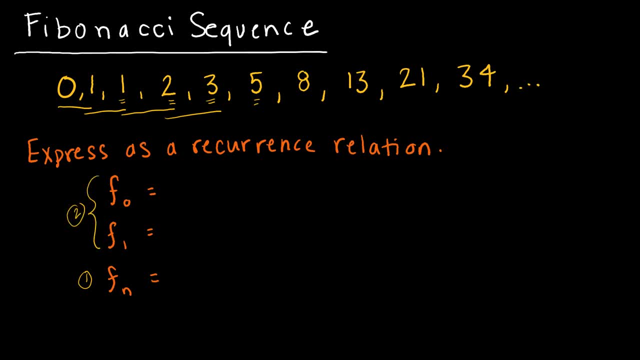 And the initial conditions. and in this case there are two initial conditions because again you have to add the two values before it. So the first value would be zero and the next would be one, because those are the first two terms in our sequence, And then the function would just say: take the value before it. 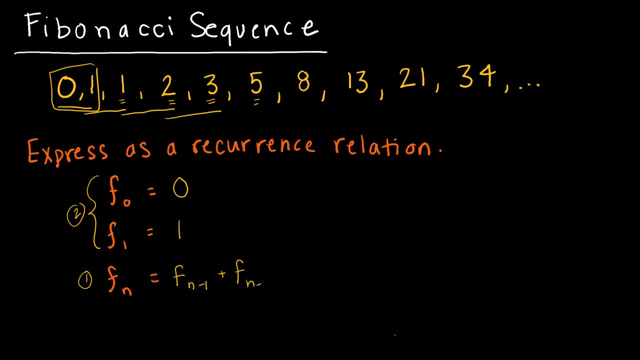 plus the value before that, And that's how we could write this as a recurrence relation. And again, what else do we have to do for this guy? for the equation we have to say for n is greater than or equal to two. 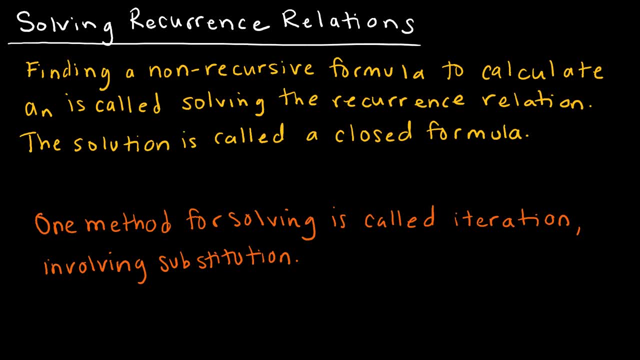 So, as we've talked about before, recurrence relations certainly have their place, but they don't have a place. If, say, I wanted you to find a 100, the 100th term of the sequence, Then this would be a real pain in the butt because a recurrence relation would require me to find all of the terms before that 100th term, And that's a lot of math that I would have to do. 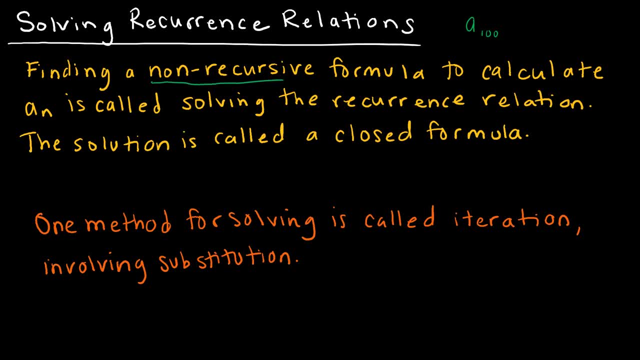 So what we'd like to do is to find a non recursive formula and explicit formula or a closed formula, And we've worked on that a little bit when we talked about arithmetic sequences and geometric sequences and how to write those in that way, Um. 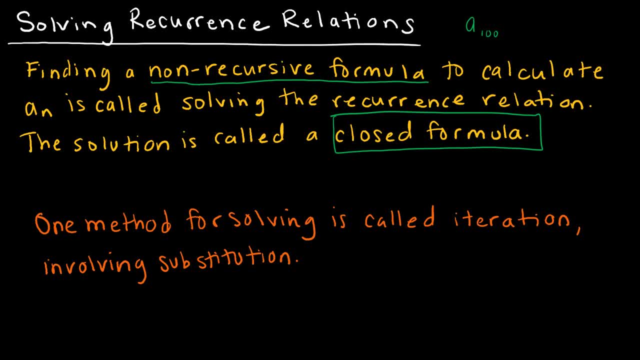 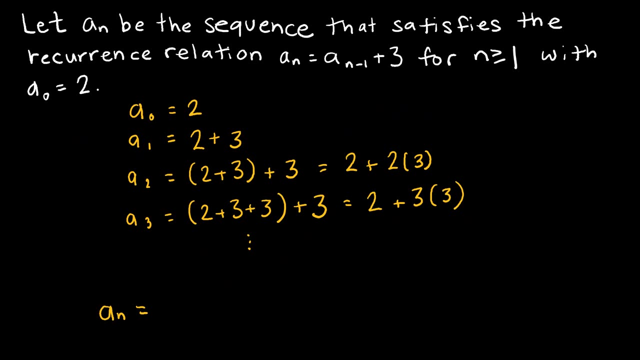 But quite often it's not an arithmetic sequence or it's not a geometric sequence. so then we have to find some other way, and One method for doing that is called iteration, and it involves substitution. Let's take a look at our first iteration example together now, before we do this iteration example, as 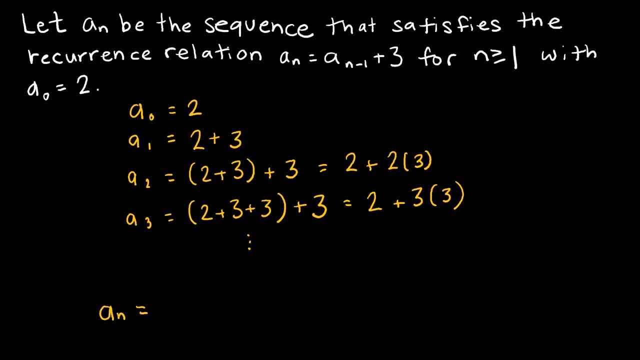 An iteration problem. I do want to point out to you that you can skip all of that work if you're very intelligent and recognize, just based on the recurrence relation, that what I'm dealing with here is in fact an arithmetic sequence, because we've already learned about arithmetic sequences and we said: if you have an arithmetic sequence, you can write that as: 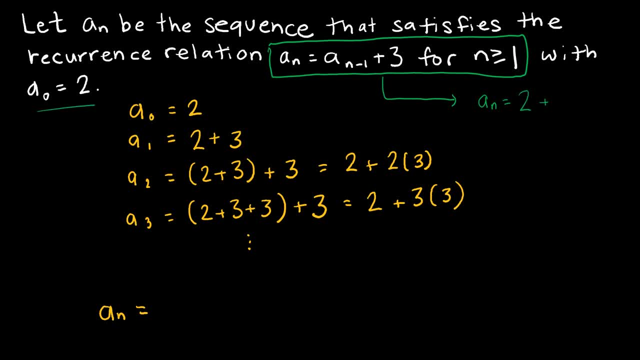 the initial value plus the common difference times n. So if I can recognize that without having to do all Of this work, then yay for us, Let's do it. But let's just say that I'm still intelligent. but I just didn't recognize this as an arithmetic sequence. 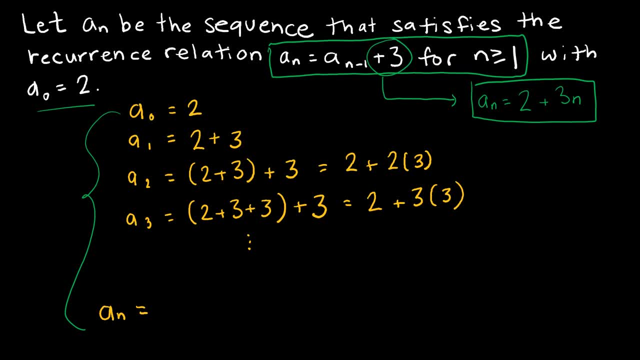 So how am I going to go about discovering How to write this function? Here's how we do it. You start with your initial condition 2. you use this recursive relation that says take the term before it, 2 and add 3, and notice I don't have to put equals 5, because 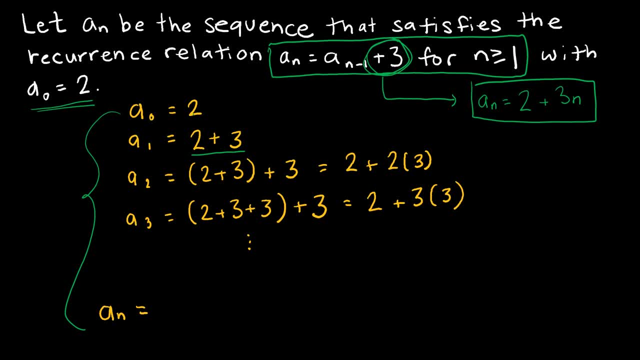 I don't care, I'm not looking for the solutions, I'm looking for the pattern To find the next one. I'm taking a sub 1, which we just said was 2 plus 3, and I'm adding 3 to that. Now I'm going to simplify that and say that's the same as 2. 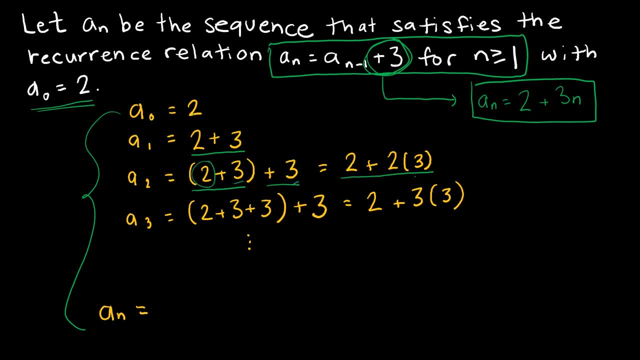 plus 2, 3's. and then I'm going to take my 2 plus 3 plus 3 and I'm going to add 3 to that and I'm going to simplify that and say this is 2 plus 3, 3's and 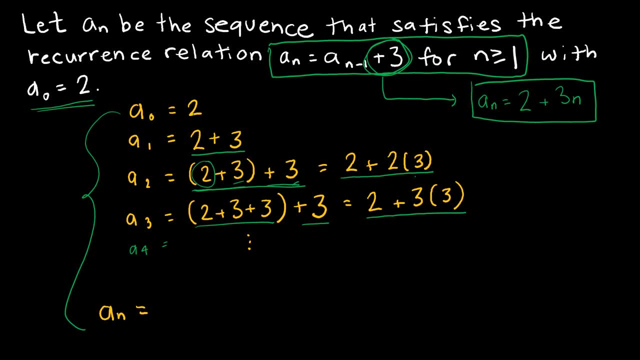 Again. I could do this for As many times as I needed to. this would be 2 plus 4 3's, and We can see what's really happening is I'm taking 2 plus n Number of 3's Which I'm going to write as 3: n, and hey, look at us. 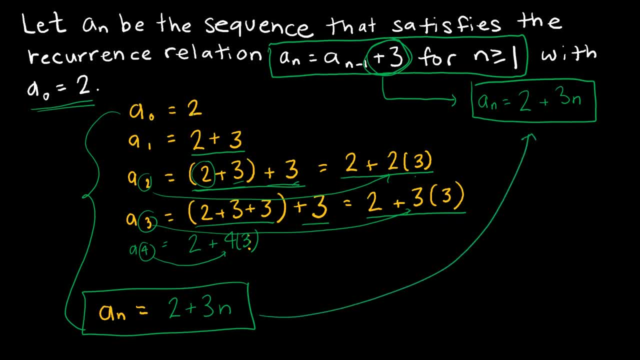 We just arrived at the same equation that we came up with knowing that it was an arithmetic sequence. but again, This is how you use iteration, is? you just write it out. You don't find the solutions, but you just write it out so that you can start to discover what that pattern is. 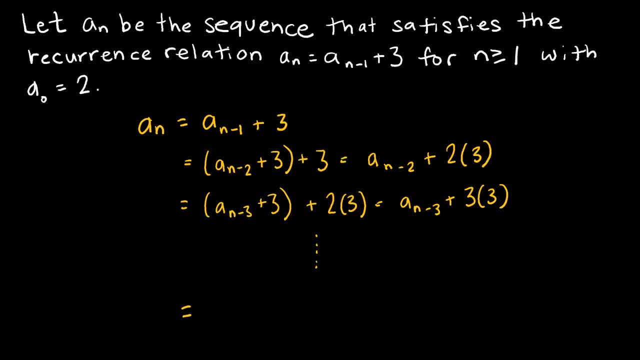 Now we're going to look at the exact same question and we're still going to use iteration. I'm just going to show you a different way to use iteration. So on the last one, we sort of went bottom up. so we started with 2 and 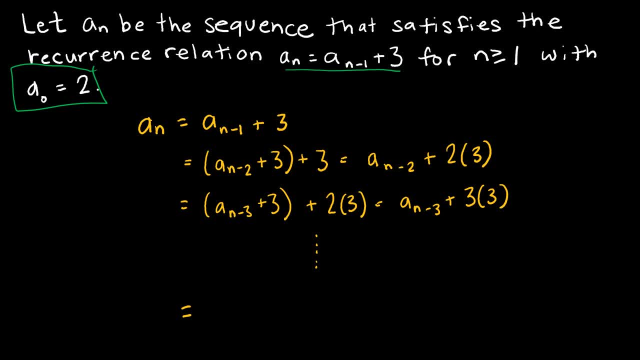 Then we used the equation to add 3 and add 3, and add 3 and then find a pattern. that way, in this method- Still iteration- I'm going to show you how to go top down. So I'm going to start with this equation and